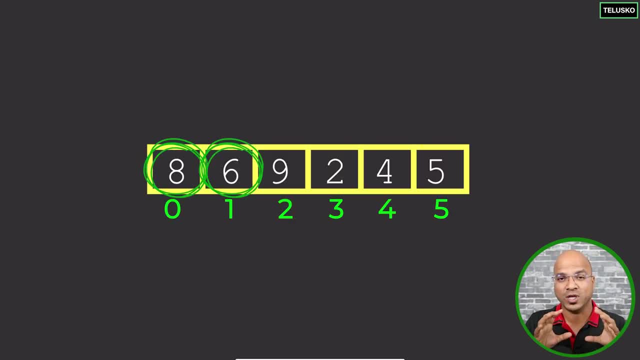 basically, till this point, when we talked about bubble sort or selection sort, we were doing the algorithm on the entire collection. so let's say, if you have a list of values, which is six values, so what you do is you perform the operation of bubble sort and all the sorting techniques which we have done before. 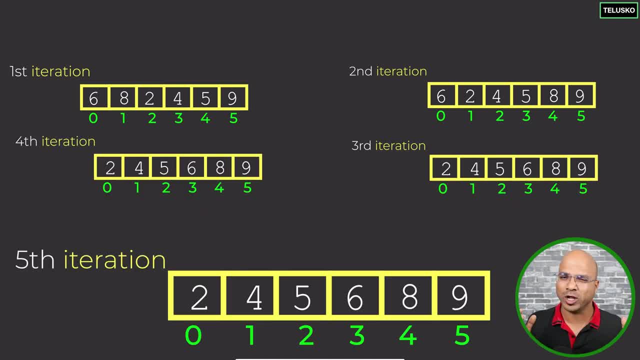 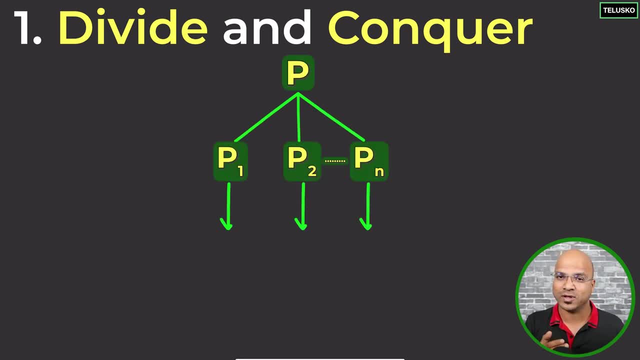 applied on the entire list. but what quick sort says: let's do divide and conquer, which simply means divide your problem into multiple things and solve the problem or sub problems individually. so what you're doing is you're dividing it, you're solving it and at the end you will combine it. so that's. 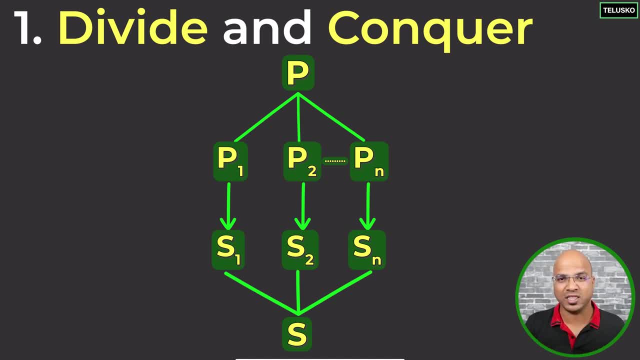 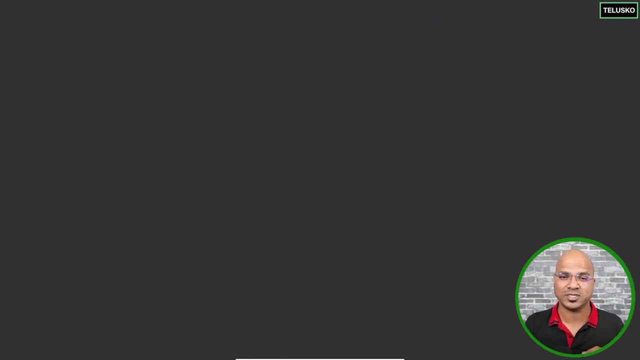 your divide and conquer. so in this case, if you have six values, let's divide the values into multiple sub problems and then sort it and then combine it. so that is your divide and conquer. Next, it uses something called a recursion. of course you can also use recursion in the other algorithms, but here it works. 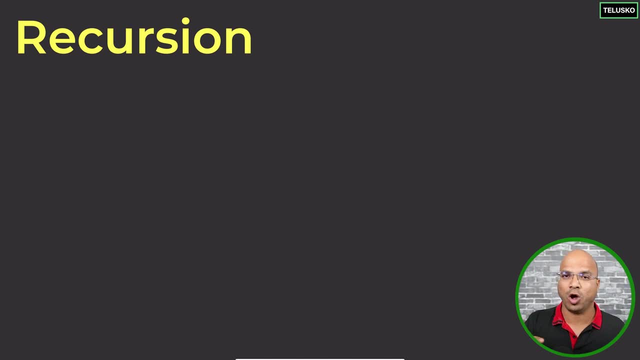 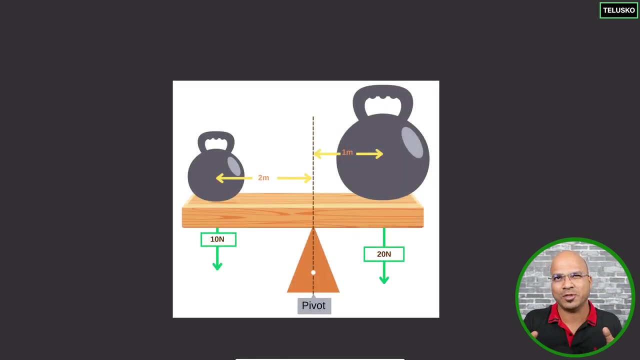 with recursion. now, basically, what is recursion? so, when you call the same function by itself, so example, let's say the function name or the method name is show, and if you're calling show inside show, that's your recursion right. and next we have to understand the concept of pivot. now, basically, pivot is something called a. 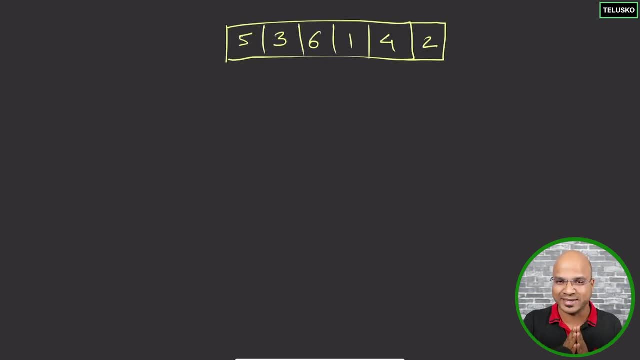 central point of a problem. okay, so let's say you have this entire list here, or the array. now you have to find a pivot and then, based on that, you will perform the operation. of course, it will make much more sense when we start, but remember, we have to work with the pivot. so those are the things you have to. 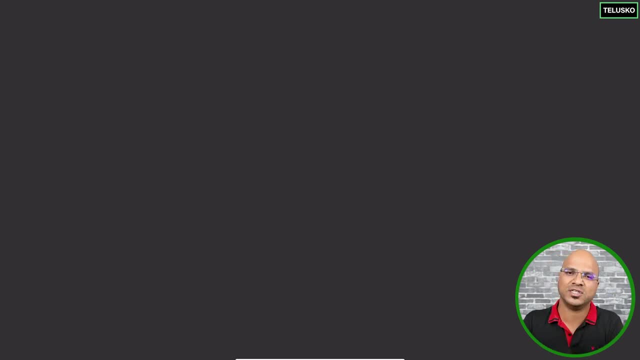 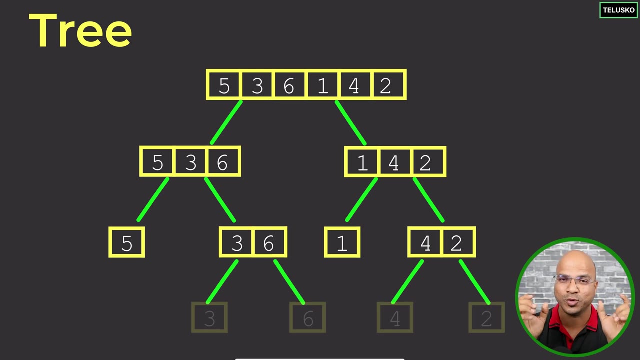 remember: divide, conquer, recursion and pivot. there's one more thing, which is the tree. now, basically, when you say you are dividing your entire list into subsections or sub problems, what you're doing is you are creating a tree structure. okay, so once we start with the diagrams, it will make much more sense. but these are the 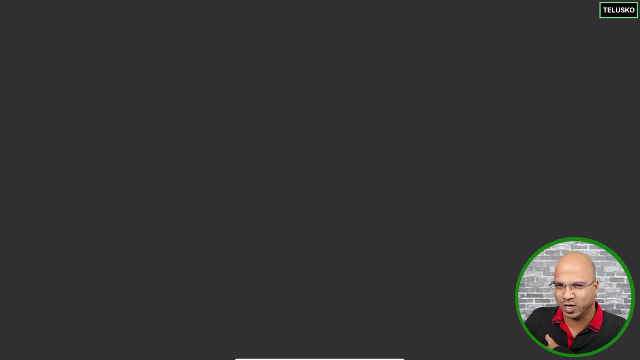 things we have to remember. so let's see how your quick sort works, and then we'll try to convert that into algorithm and then we'll see how to write a code for it. now, the basic idea here is: let's say, you have a list of value, so we are discussing about quick sort. so let's say we have a list of values and we're going to talk about it briefly. So what we have here is a list of values which we already know about. but let's say we have a list of values which we already have. 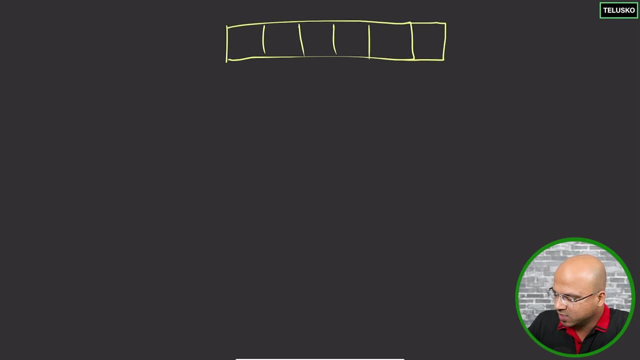 values. so let's go for six values here and I will say: this is five, this is three, six, one, four and two. so let's say we have the six values. I'm not sure will it really make sense to use this example, but let's get started now with this six values. what you normally do is you do divide and conquer. 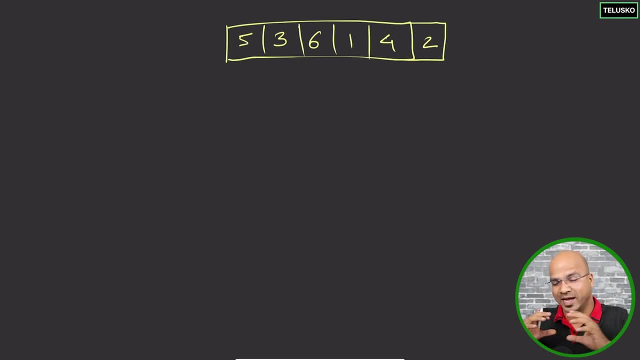 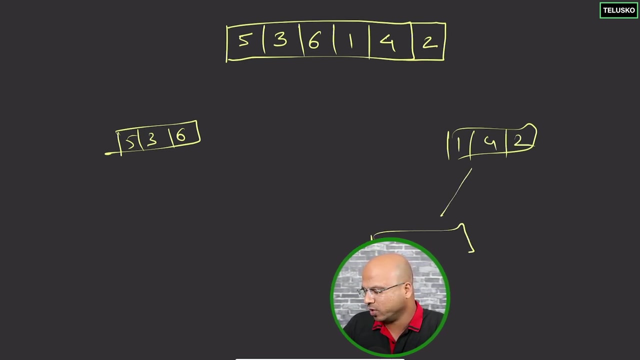 here. so the basic idea is break the entire list into sub problems. okay, something like this: maybe we can create two different, two different arrays. here we'll be having three, I mean five, three, six. here you can have one, four, two, and then you can again divide this. maybe you can have one and four. 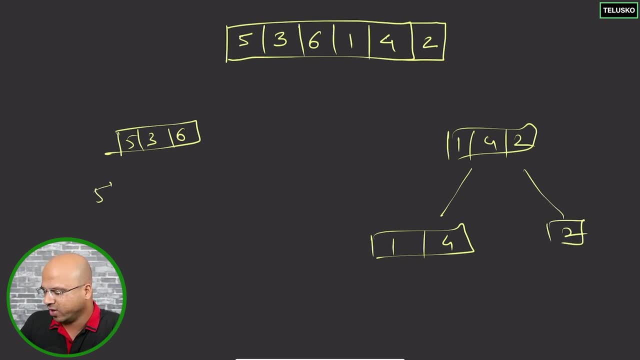 here and divide this into two. here also, we can have five, and then we can have another array which is three and six. so we got these two arrays from the big array and then you create the shorter format of it. so at the end, what you're doing is you're getting the small chunks. now. this is what. 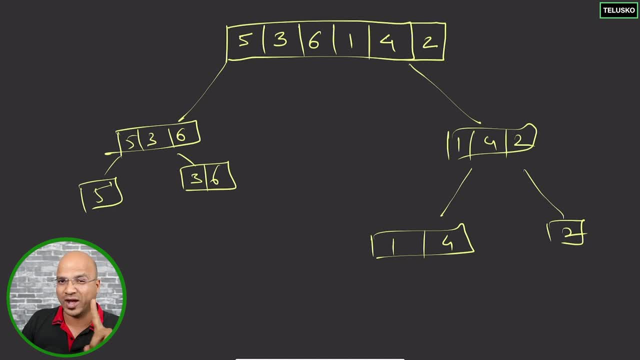 you're doing is you're creating the smaller format of it. so, at the end, what you're doing- tree structure- is so we have divided, we talked about dividing, so we are dividing it. we'll sort the array and then we'll combine it and then, since we are performing the sorting on each, 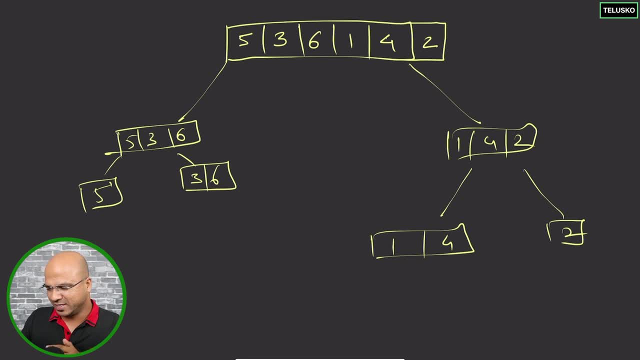 section in sub problem. that is your recursion, but is it the real thing? no, so basically, we talked about the idea, but how do you divide the array? randomly? I just divided the array, but that's not the main idea. but we have to divide, but not this way. so how we are going? 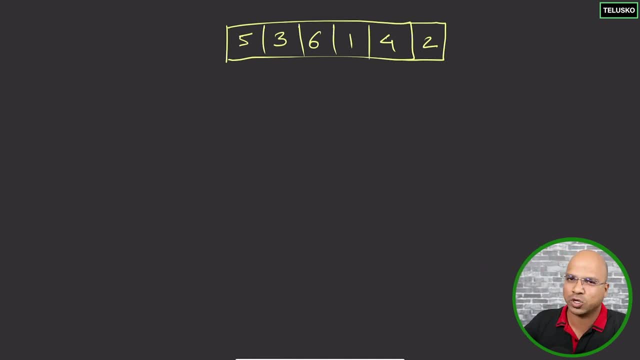 to divide this? that's the question. let's remove this and let's go with the values. the idea is: you want to divide- for sure you will divide this into two parts, but you need to find a point from where you will divide this, and that point is basically your pivot. now, how do you find? 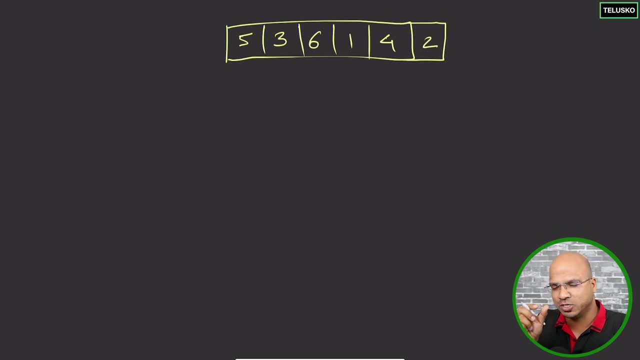 a pivot now, basically the reason we get this partition or pivot to do the partitions of the array right now. should we pick up one now? that depends. so even before you divide you have to do one more thing. so I'm saying pivot, but then that pivot should be a point which is at the right. 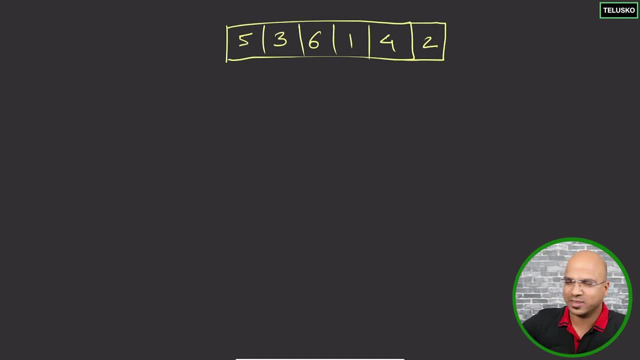 position. let me repeat: the pivot is a point in this array which is at the right location now. if you see this, after this, sorting what the values you will get. so you will get values like, let's say- I will just write it in shorter format now- so you will get one, two, three, four, five, six. this is the. 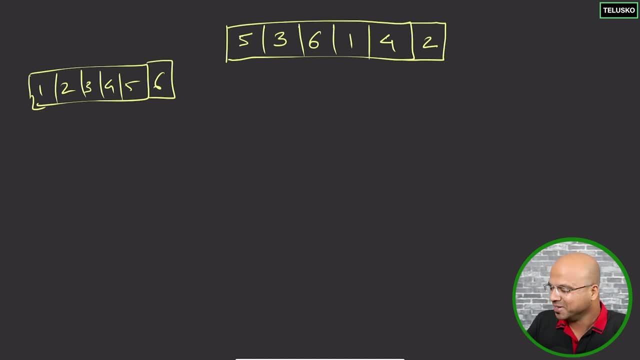 output I want. okay, just wait for the sequence of numbers here, but this is the output. so this is the output which we want from this input, which which we have the bigger array here, or the big size which we want from this input. okay, so if you talk about the value one here, so one should be at the first. 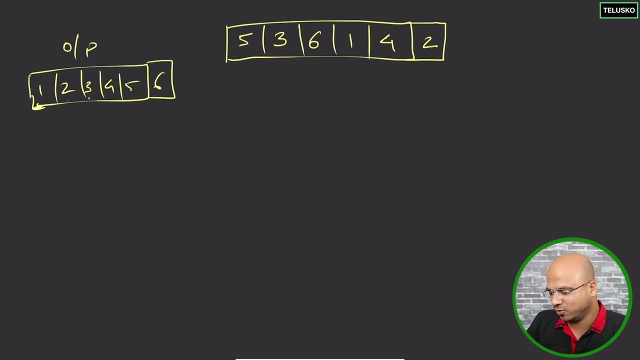 position two should be the second, position three on the third position fourth, fourth position fifth, fifth and six right. so they should be at that position now, since we have taken those values, and that's why it might be confusing. but you got the point right. it doesn't matter what your values. 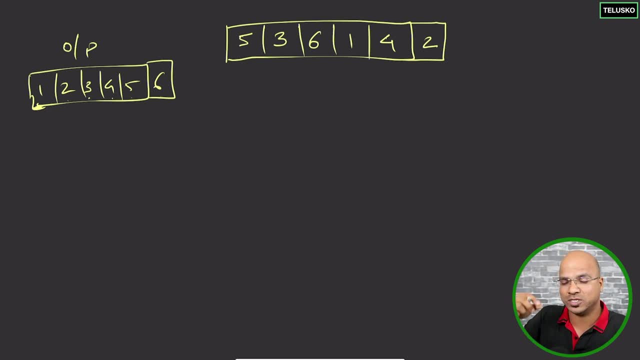 you have. it should be in the ascending order, so the first value, the smallest value, should be first and then at least goes on. okay, now we have to make sure that at least you will you find one point from here or one value which is at the right position. example, if I say: let me, let me take four, now four. 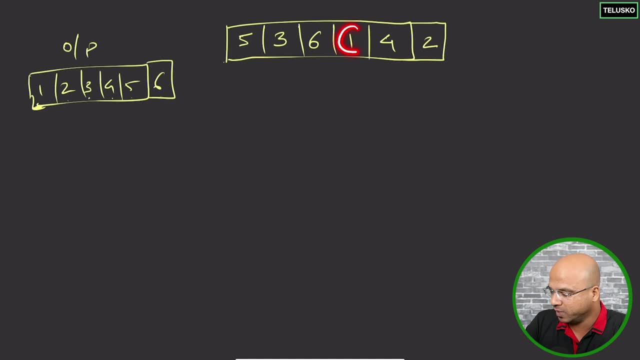 is it at the right position? the answer is no. four should be here, right. so instead of one, it should be four. then we can say four is at the right position. now, if you want to understand this with an example, so let's say you're in a classroom and then you have multiple students there, okay, and 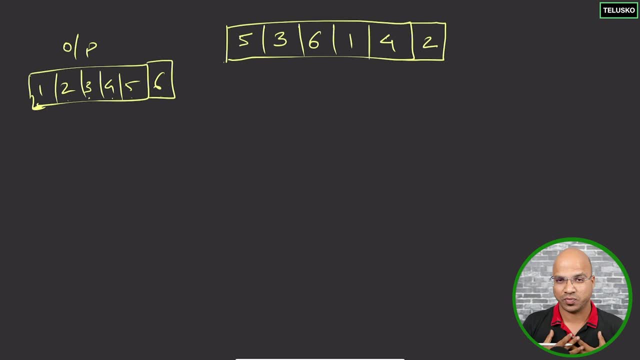 then you want to sort them based on their height. there is one way: as a trainer, I can be there and I can say: okay, you go there, you go there, and that's what we have done in the bubble. sort right, I was controlling it. but what if student can sort themselves so they can compare each other and they 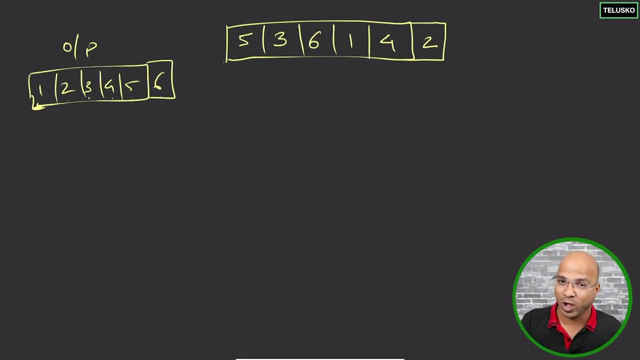 say, okay, I should be here, or I should be here and they, they will move. now one way is one person can sort them, but then we don't want it. so what we want is what if the students themselves can get into the right position, that that will solve the problem. right, okay, but how we are going to do here. 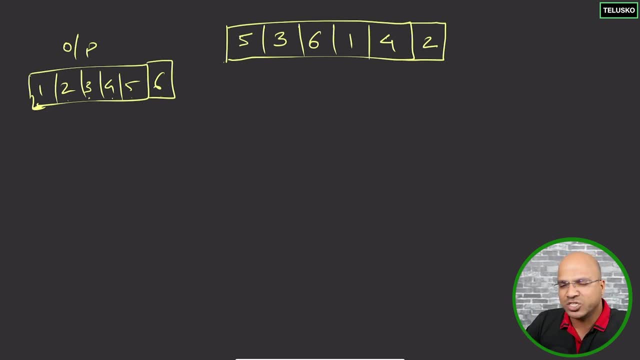 how they will reach to our right position. now what you do is, initially we don't know the position right, so you can take any value, normally we can. we can find the pivot. so for the first iteration we what we are trying to do is we want to make sure at least one value is at the right position so that we can divide the array. 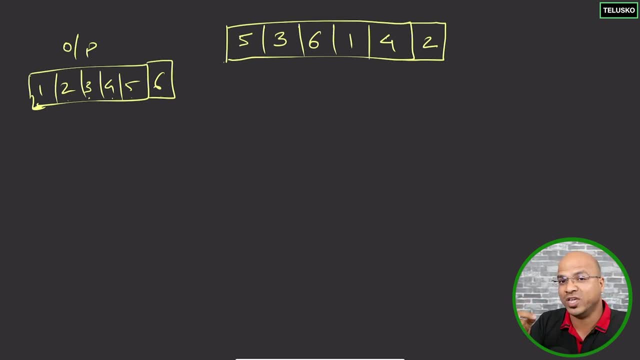 now, which value should we take technically, if you take the average value, or if you take the middle value? example, if you, if you go from one to six, the mid value is three or four. right, so if I can take three as my pivot, it will be much easier for me to divide the array. so what will happen is, if I take 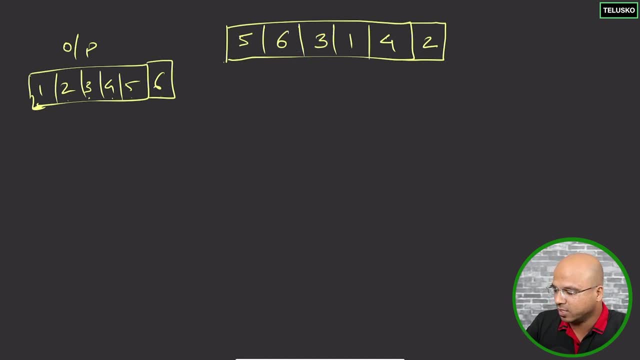 three should be coming here, right, so three: this is the right position for three, right, but it's not. if you start with the area, this is not at the right position. but if you get to the right position, we can divide into two parts, right, okay, so that's the main idea. how will you get that there? so normally? 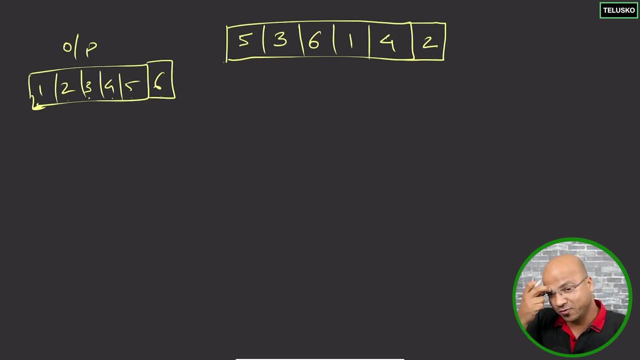 what you do is if you can find a good pivot, and that's very difficult to find, because how do you know the mid value? since we know the values here, I can find the mid value, but as a program or the software, they don't. they don't have any idea what are those values are. so what we do is we randomly 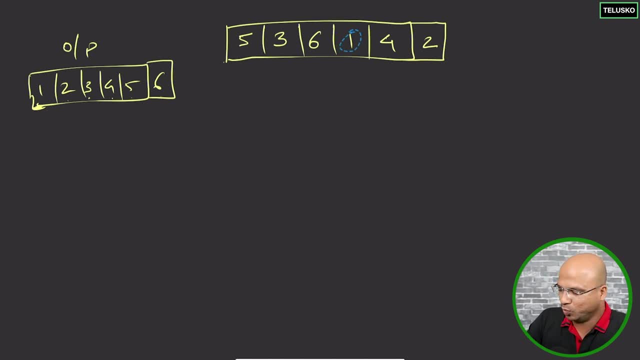 pick the pivot. maybe you can pick up the pivot, let's say one in between, somewhere, anywhere if you want. so you can pick up this one, you can pick up the six, or you can pick up the first value, or you can pick up the last value, or what you can do is you can, you can just add all these values and 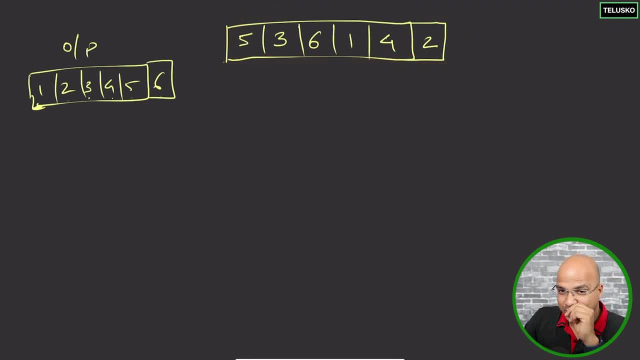 divide by six whatever value you will get. so try to find the average of it. that's what we can do, but again, that's a lengthy process. normally- which I have seen- is they go for the big, the last value, not the biggest one last value, because we don't have any idea what's the biggest value. 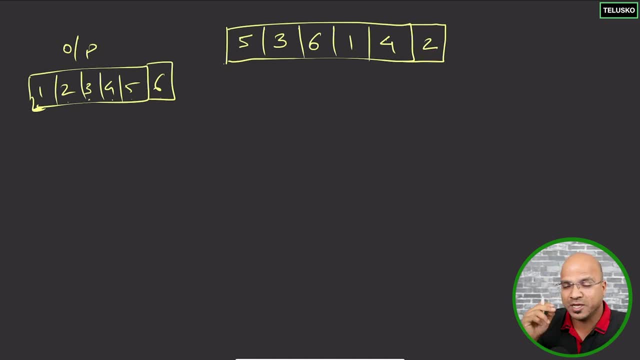 is. so we'll go for the last value, okay. so this is: this becomes your pivot. that means we need multiple variables here. now what variables we need? so we'll just write variables here. so the first variable we need is a pivot variable. so we'll say pi, okay, and then you need few more. 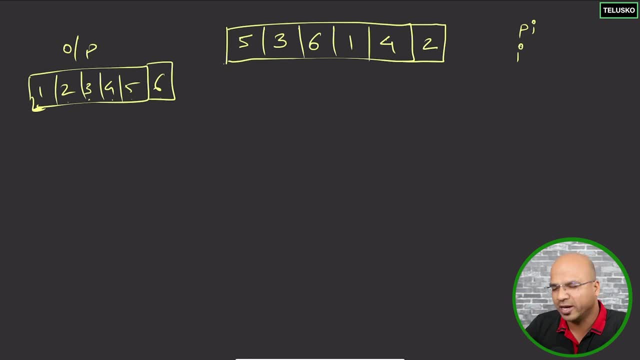 variables. you need a variable I for the positioning- again we'll discuss what this positioning is. then we'll need a J which will track, which will go through each element, and we have done that in the sorting right. so when, when you jump from each value, that will be done by J. and then, of course, we 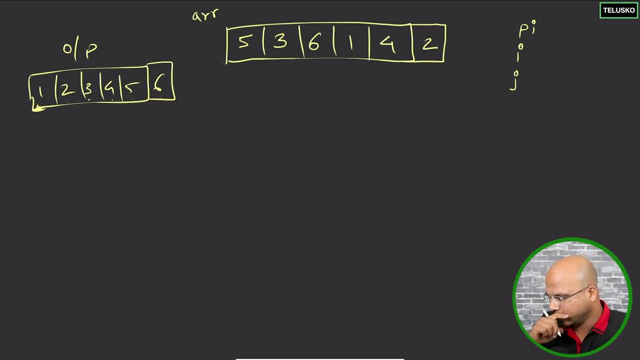 also need array here. so let's say: this is ARR, this is your array, okay. and let's have the index value. so we'll say this is zero, one, two, three, four, five. those are the index values we have. apart from this, we also need a low and a high variable, okay, so it will say L and H. so let's say this is L and this is H. now 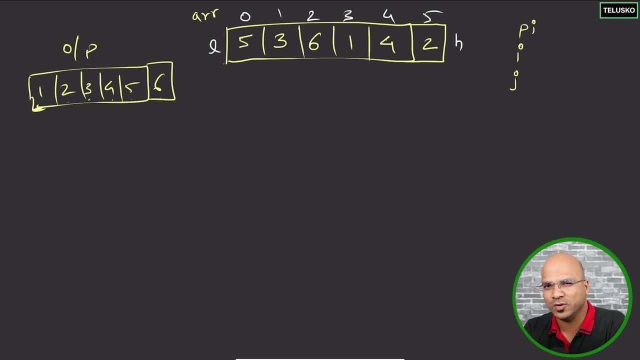 normally we can say H is the last value, or we can say it's a length minus one. so we can say that. so we have a low and we have a high. so low starts from the first. H is the last value. now how do you perform the operation? it's very simple. first you find the 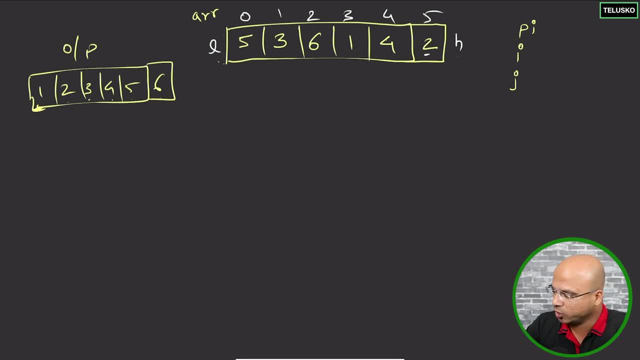 pivot. now we know that we are going for pivot, which is two in this case. so what you will do is: let's take this two as the pivot, so I will say: this is P, so this is referencing. this is referencing this two, so P- I variable at this point is referring to. so I will say this is two in this case, and then 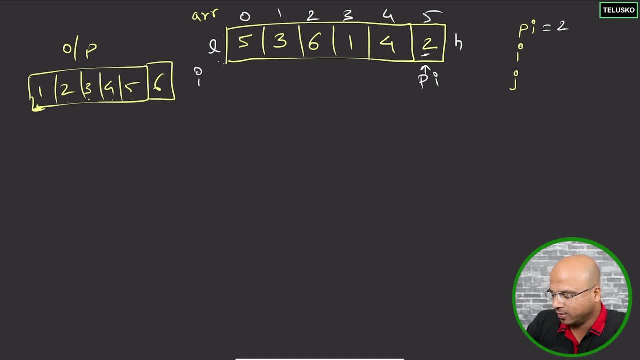 we need two variables. so let's take variable I. now, by default, the value for I will be the lowest value one. so let's say the i value is here at this point. you know what i will do. let me just remove this portion at this point because let's keep this slate clean. so we need an i variable and then 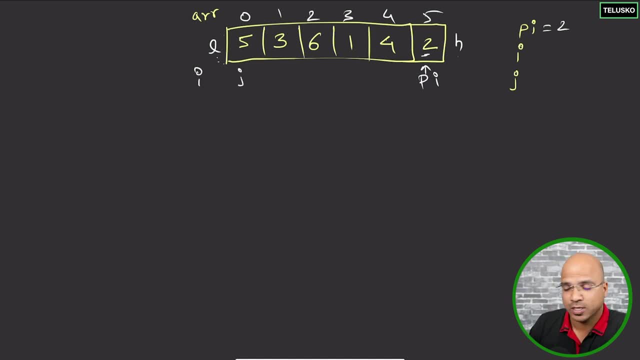 we need a j variable. so j will be here to start with. so i will be here at the minus one position, j will be here at the zeroth position, and then what you do is you basically run a loop where, of course, the i will also increment, but the main loop here we want is for j. okay, so we'll take a. 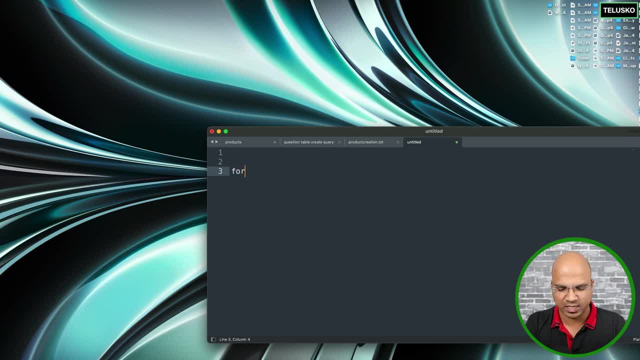 for loop for j, okay, so let me write the code here. so what we want is, of course, the rough code. so i will say: for j will be starting with low. okay, that's what we are doing here. and then j should go till n, but then we are not using n variable, right, we are using variable high. so let's say: 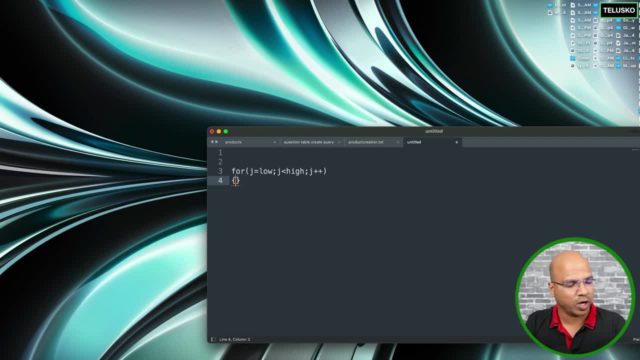 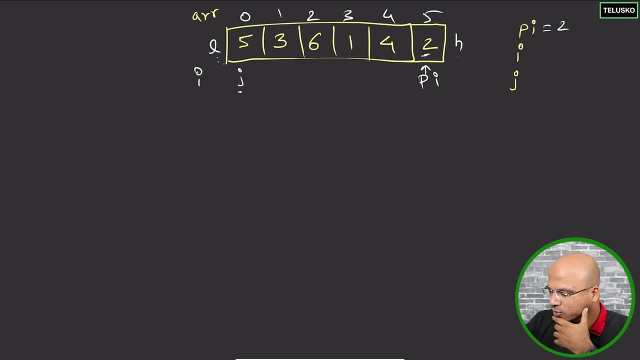 j less than high and j plus plus. now what you are going to do in this, inside this loop? so, basically, you will first make sure that you get the pivot value right, so you will. i mean, of course, you have a value here which is two, and then you also got i- i is still minus one. now, inside this loop, what you 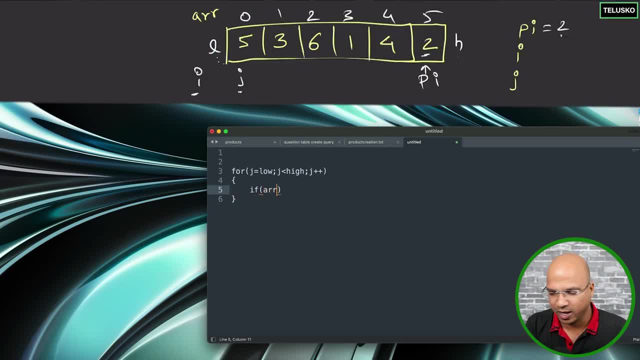 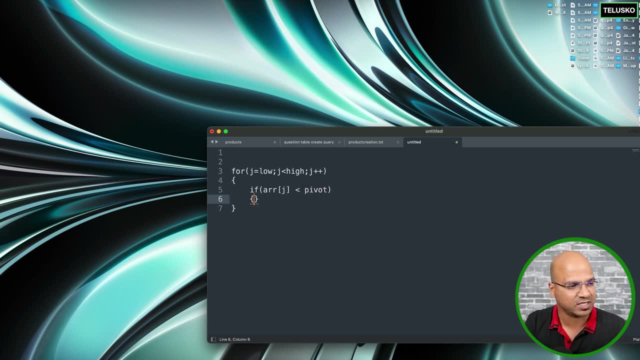 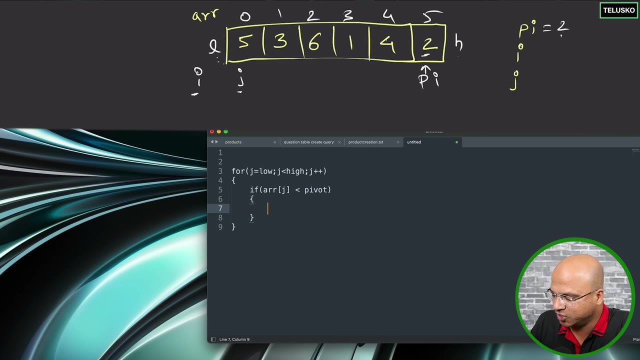 will do is you will check if the arr- which is in this case we have an array- if arr of j, if it is less than the pivot- so pivot, we have a variable here- if it is less than pivot, you will perform some operation. now, if you compare the values here, do you think the arr of j, which is five in this? 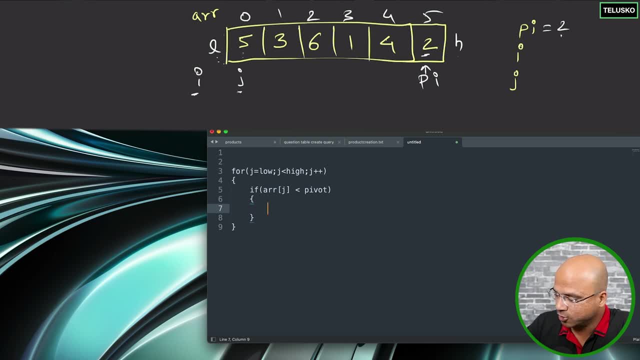 case. is it less than the pivot, because pivot value is two. no, it is not less than uh pivot, so we'll not do anything, but we have to find the value which is less than two. right, so if the value phi is less than two, you will perform some operation, it is. since it is not true, we are not going to perform. 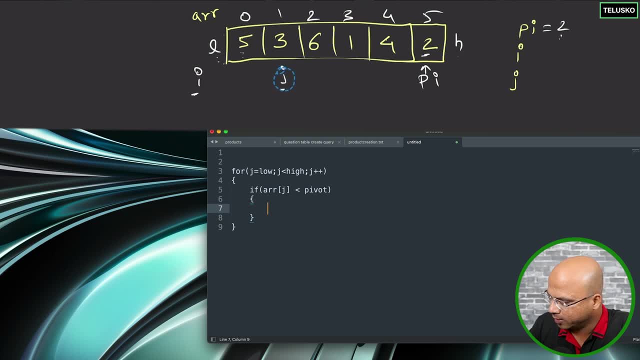 any operation here. so basically, you are going to shift your j here. okay, now how? why we are doing it. of course we are running a loop, right. so j starts with low and then we have to increment. so j goes there. it will compare itself with the pivot. is it small? no, so again, you will shift your. 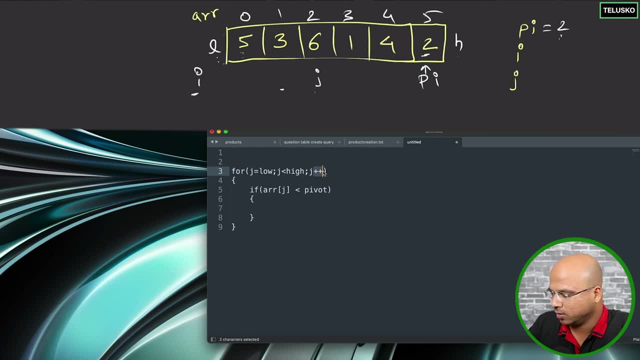 j. then you compare six with two. then is it smaller? no, then you shift your j here. then you check: is it smaller? yes, what if it is smaller? then what you will do in this case: if it is smaller, you perform some operation. first thing you do is you increment the value of i, basically what you're. 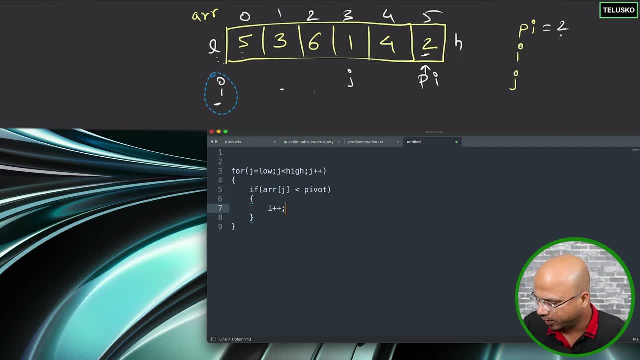 doing is you are shifting your i here. okay, that's done. next, we have to make sure that you swap the value of i and j. okay, so whatever value you have with i and j, you basically swap them. so what i'm saying is: take this value here, move this value five here. 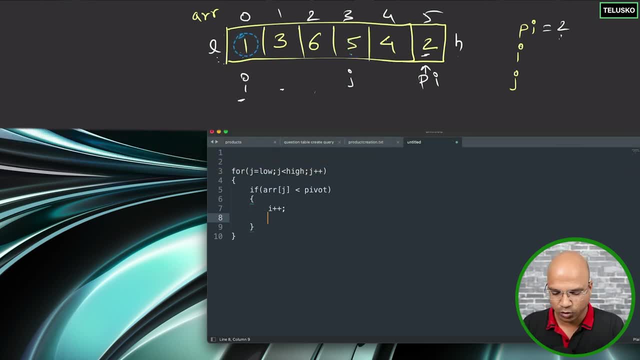 and move this one here. okay, now how do we do that? of course we have used it before, so we can use a temp variable, or maybe at this point i will simply say swap and then we'll write the logic later. so i want to swap, basically, the value of arr of i with arr of j. okay, so we need to do the swapping. 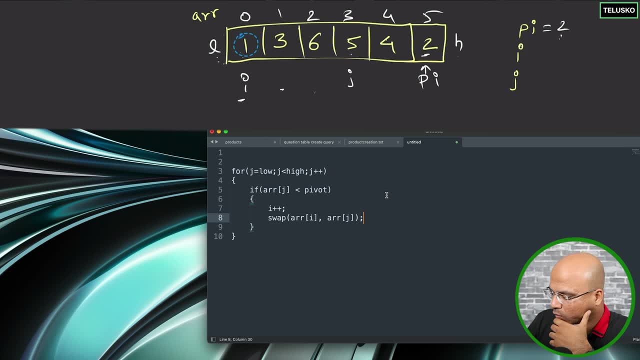 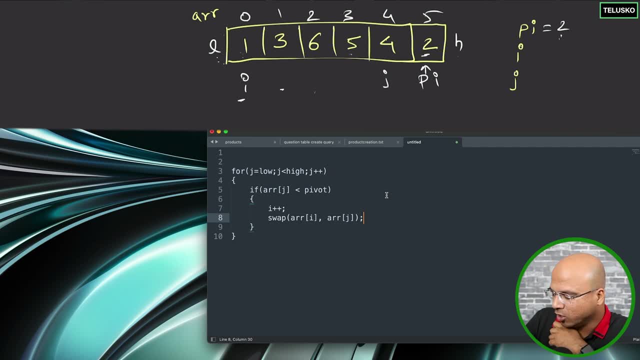 because we are in a loop. so j will go here now again. you will compare. if the 4 is less than 2, no, and that's it. j will move here, because if it is not less, then we are not doing any operation. then your j goes to the last value because your j ends at high right, so j reaches here and, of course, the 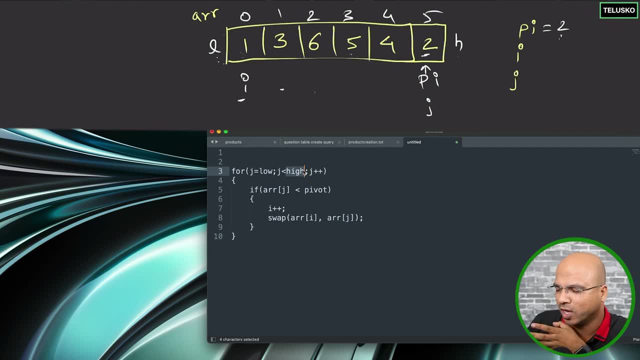 pi and j is same, then you don't. you don't have to. i mean, of course it is false. the condition this condition will be false, which is arr of j is not less than pivot. so in this case it will not swap. but what happens after that? even if you complete the entire loop, do you think 2 is it the right? 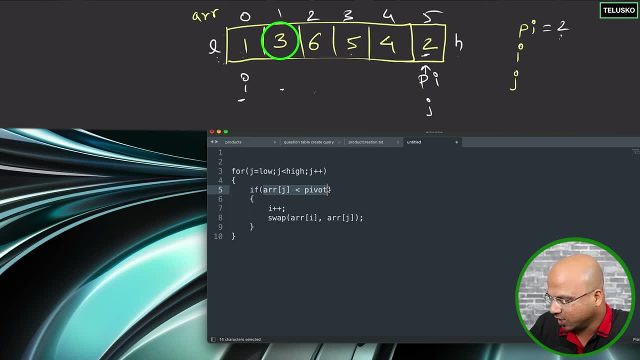 position no 2 should be here, right, so this 3 need to go there. so what you do is you perform one more operation after the loop. so after the loop, you, what you will do is you will basically swap the arr of i plus 1 with the arr of high. okay, now this is the operation you have to perform. 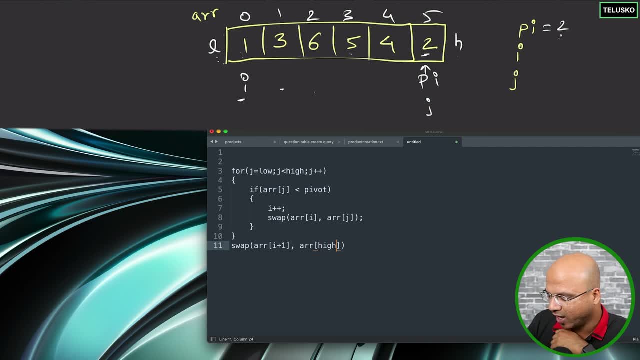 now what will be happening here? so what is the value of i? value of i- 0, which is index? you are picking the next value, which is 3, so you have to swap this 3 with this 2, because that's what your arr of high is. so you will move here and you will move this side. now, by doing this, we made sure. 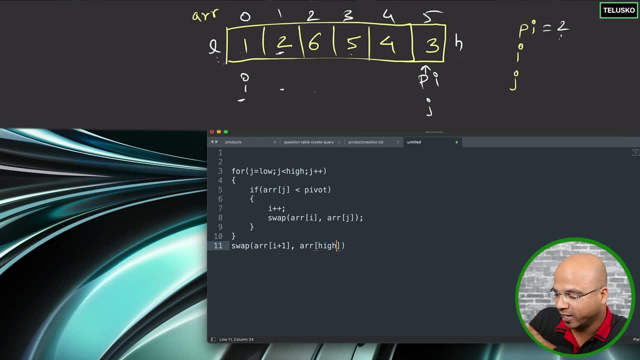 that the pivot value which you choose is at the right position. can you confirm? is it the right position? yes, it's at the right position. now, what you do is you divide. i mean, if you, if you observe the array, if you look at the pivot i, which is pivot here, now, if you see the left hand side of it, this is always lower than 2. 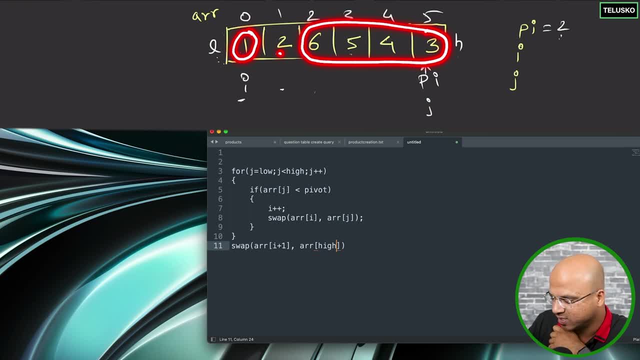 and this value is always greater than the 2. so, yes, 2 is the right position. now what's the next step? the next step is very simple: you divide this array based on the pivot value. so what you do is you create another array here, and in this you will be having only one value, which is coming. 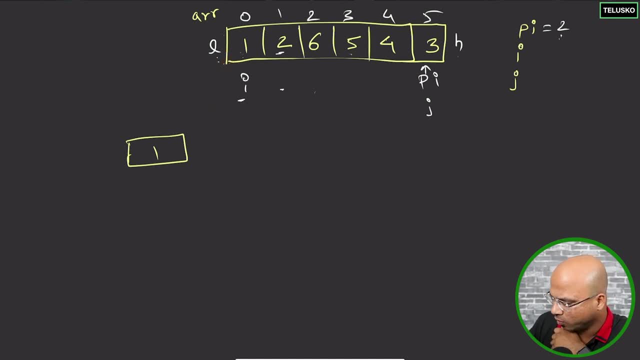 from here right. in fact, we can also draw an arrow there. so this is coming here. 2 will remain there. we can write 2 here. we don't have to work with 2, because it's already sorted and then you take this particular section into another array- not another array, but let's say logical partition. we 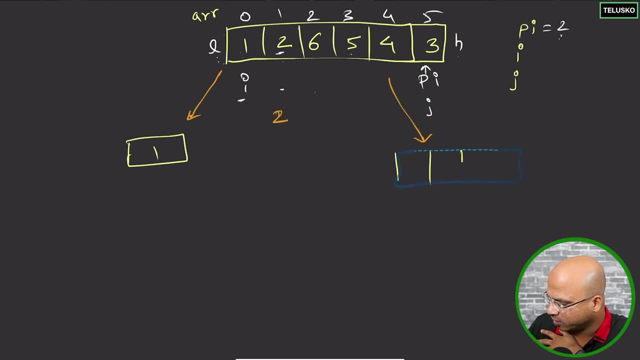 are doing here, so we'll get another array here. so we are doing divide and conquer, so here you're going to have 6, 5, 4, 3.. if you observe, they're not sorted, but at least we got the partition right now. what you do is you again perform the same operation which we have done here in the first example. now, 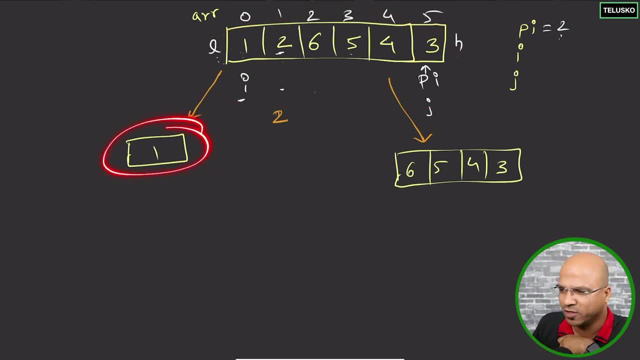 we start with this? yes, we can start, but you don't. you think we only have one value, and whenever you have one value, it is already sorted. let's work with this. so what you do is you again take the same thing, so you take the low, you take the high, and then you, of course, you again have this p of. 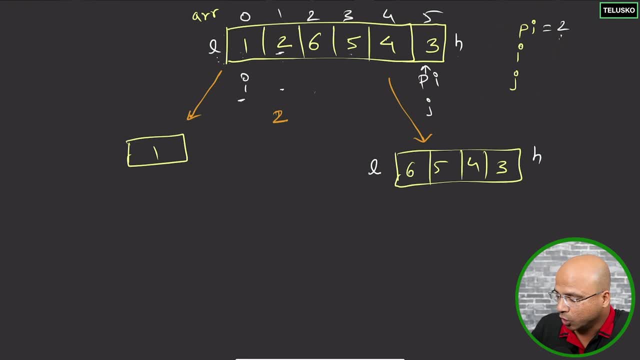 all these values here, so all these variables are still exit because you are going to apply quick sort again on this particular values. so let's get started. let's take pivot. which pivot we are choosing? of course, we are choosing always the last value. so this is your p. 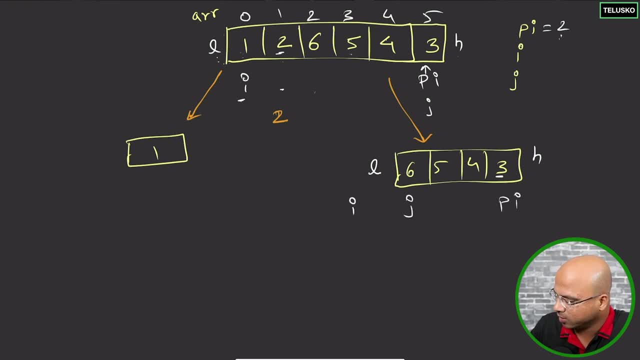 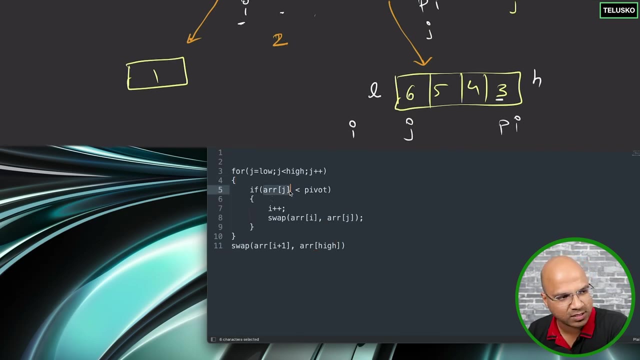 i pivot. then you got i here, you got j here. then what you do is you start running your algorithm, which is: first, you compare the value of j, which is 6 in this case. is 6 smaller than 3.. look at the algorithm which we have done: is 6 smaller than the pivot? the answer is no, so you will simply: 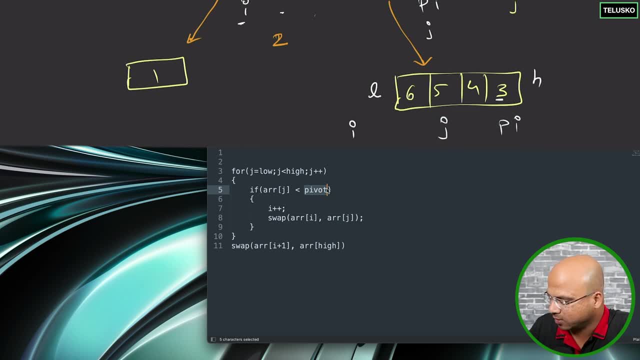 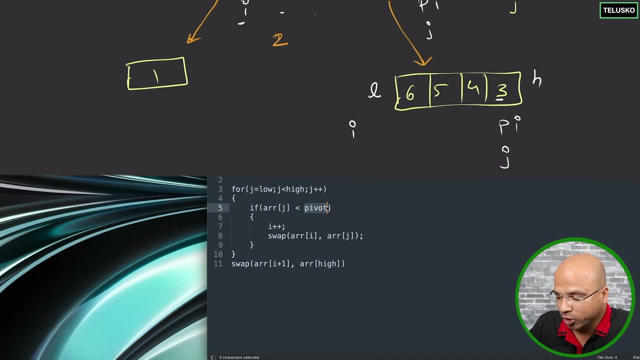 so you will simply move your j here again check: is it uh small? no, shift, is it small? is it? then again goes here: is it small? no, then what you do is: you have not. you have not done any swapping, but at the end we got one more logic right. so once you complete this for loop. 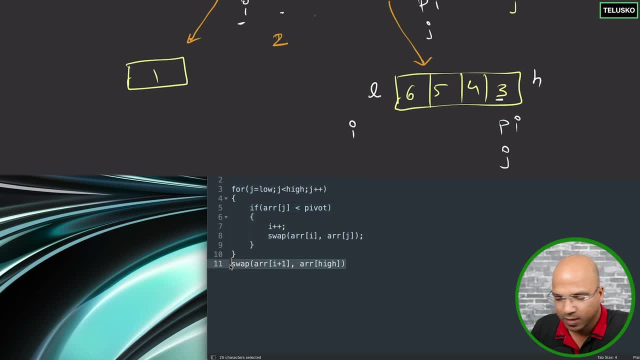 you will do something with this, which is swapping the i plus one. so i is at minus one. so you have to basically swap the six with the area of high, which is three. so this goes here and this goes here now. if you look at the pivot, this is sorted right. so now. 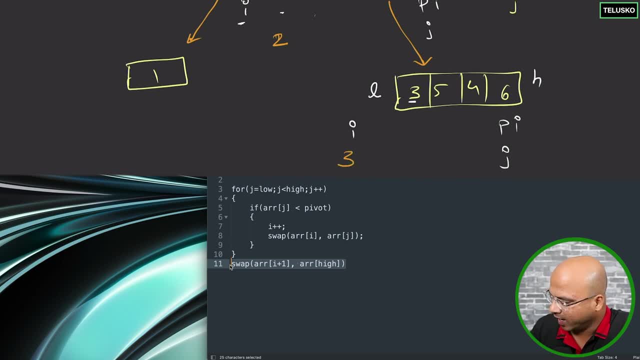 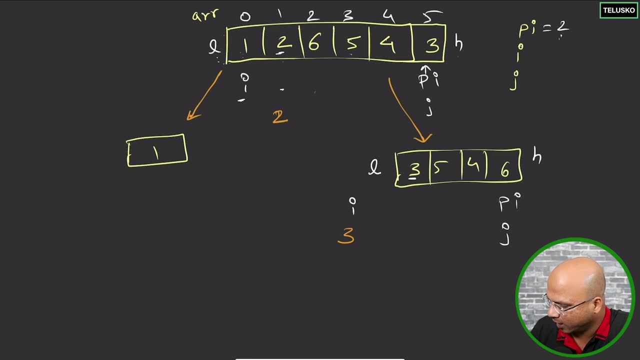 you do is you write three here, which is your pivot value, and then you divide your array into two parts. but since the pivot was the first value, what you will do is you will get the new array now from this, which is five, four, six, and then you start performing operation here. 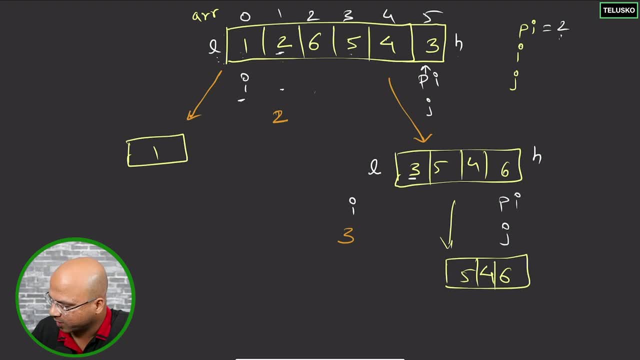 now, what operation? the same operation which we have done again. you will apply quick sort, so this is l, this is h, so pi is referring six here. and then you start: so you got i here, you got j. then you start comparing. is the first value, the value of j? is it smaller than the pivot? yes, now 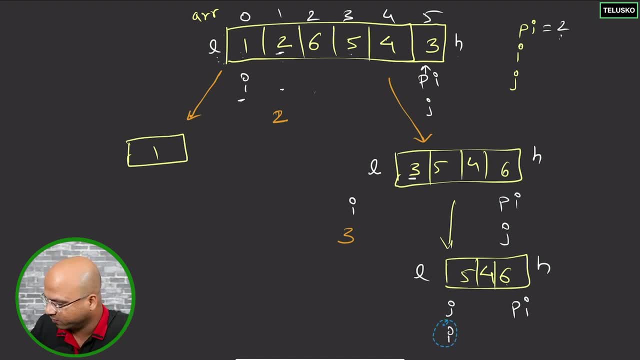 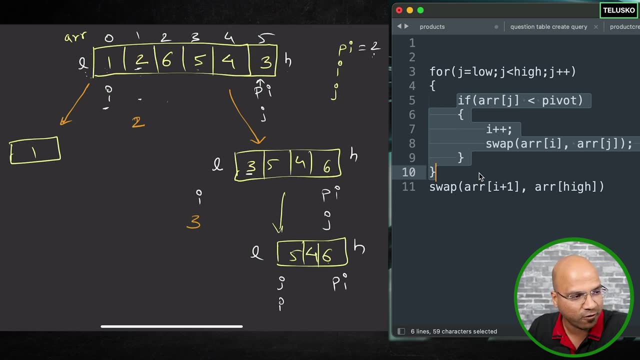 when you say yes, what you will simply do is you will increment the value of i first- if you look at the code, that's that's what the logic we have- and then you swap the value of i and j. now, in this case, i and j are referring to the same value, so swapping doesn't make sense. of course they will. 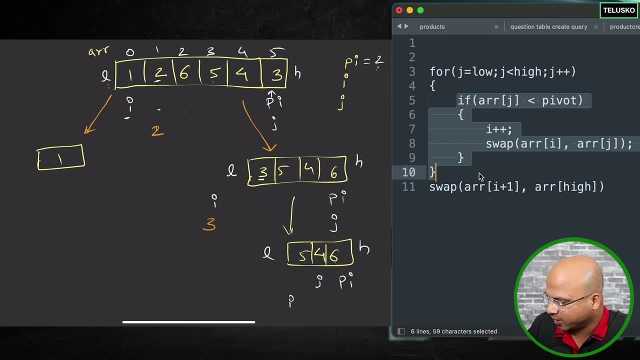 get the same value. then you increment the value of j. j goes here. check is 4 less than 6. yes, in that case you can move i here and then you will swap the value of i and j again. it remains same, so nothing to do here. then you shift your j. here, of course, the array of j is not less than pivot. 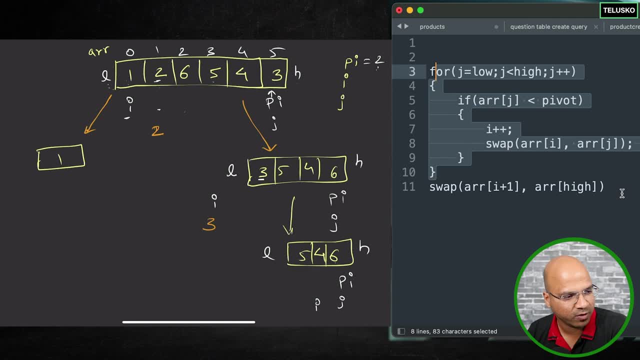 because they're the same value. then this loops end, the for loop ends. then you perform this operation, which is arr, which is plus one. this will be replaced by high and that remains same right. so there's no swapping. i know it's all depend upon the value, type of values you're. 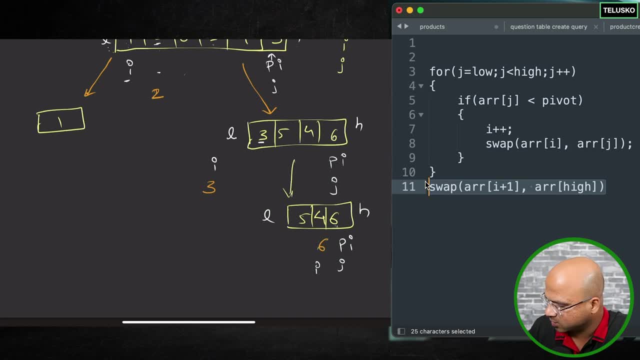 getting so. at this point there's no swapping happened, so this remain as it is- six. but then you will get a new array here which only has five and four, and then you start applying the same operation. let's get started. if i will just write this bit. 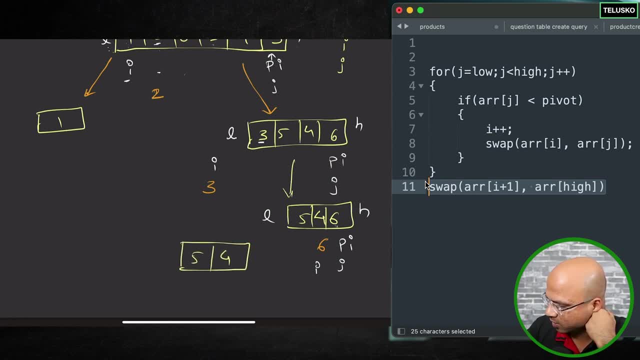 up so that i will have some space, and this is coming from this particular section- then what you do is you will take the same value, you say, and if you observe we are doing recursion right, the same steps, we are repeating multiple times. so l h, we got p i here, we got the variable i referring. 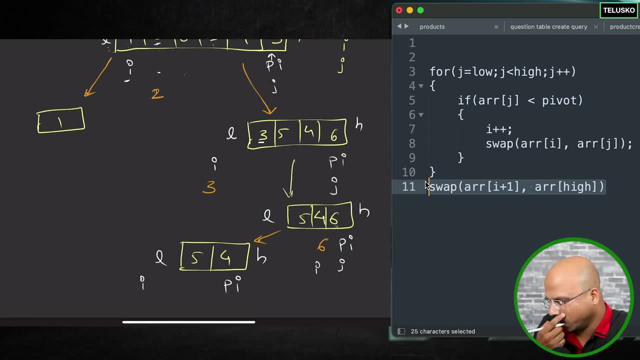 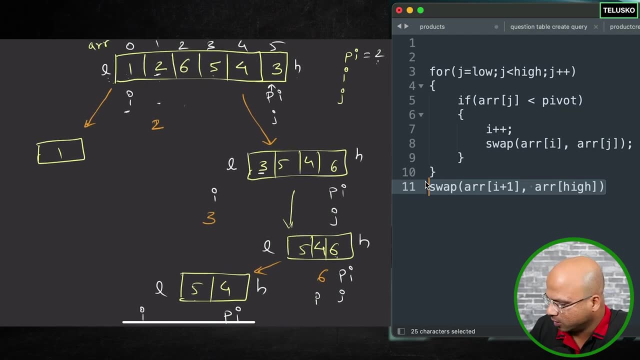 to minus one position, or, in fact, not minus one position, it is one less than the low. so, in this case, the low is this position right now. what is this position this is? in fact, we should have maintained the index value, right? so this is zero. this is one. this is two, three, four, five. 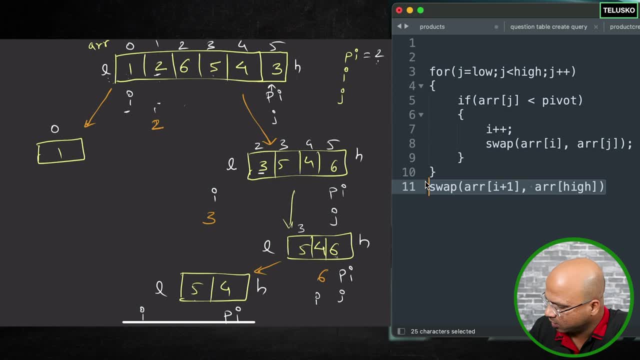 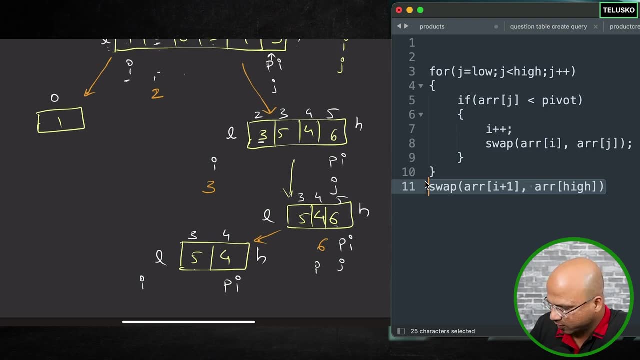 then we got three here, which is this one. this is three, four, five. what we got here is three, four. so these are the index values for them. okay, so we got- i referring to the index value- two. j is here. then what you do is you simply compare the same steps we have, which we have done, so the